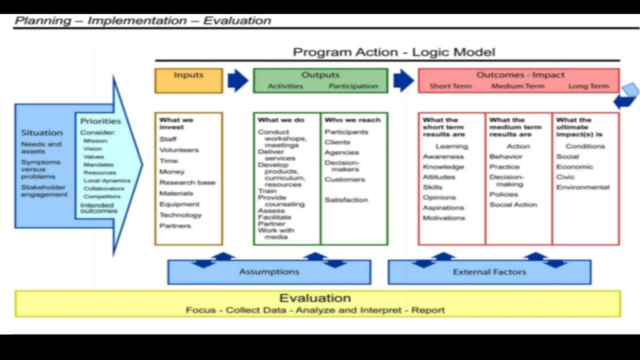 A logic model is a powerful tool and framework to use when thinking about a program's impact. Now, the word program is often used in the non-profit field. However, it can also be applied to the for-profit field, And the principles of aligning your inputs with your results is 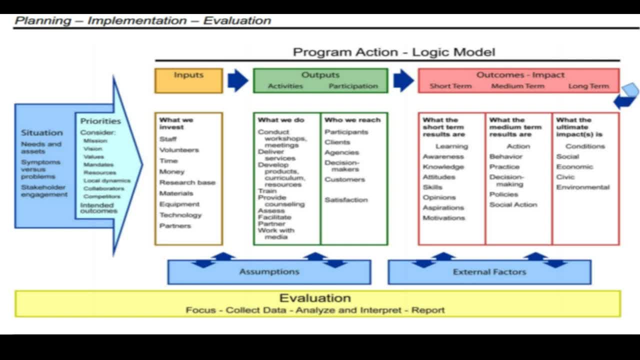 something that is applied everywhere right, And so what I want to do in this lecture is talk through some of the basic components of the logic model. I do have logic model courses that go into each component, but I want to just talk about the overview of 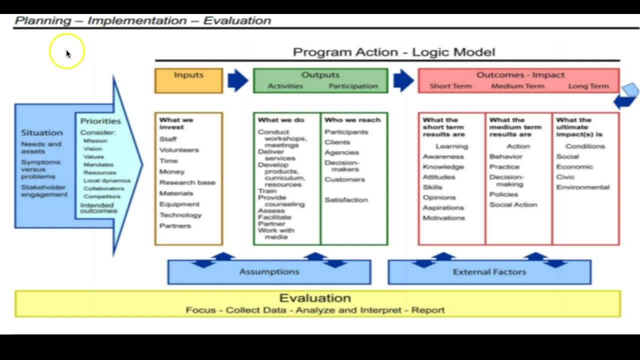 the logic model, And the logic model really is about planning, implementation and evaluation. right, We can't evaluate something unless we understand the framework that's being used. So let's begin. We have a situation where we have a program that is being used. 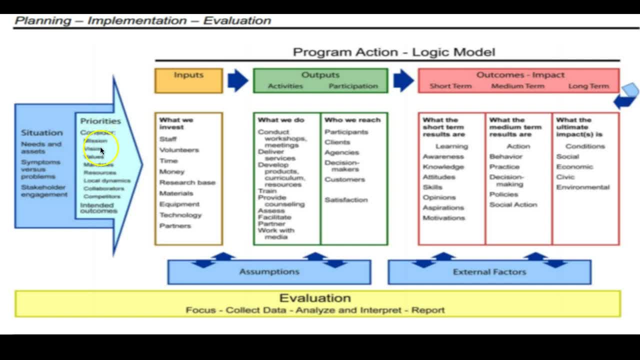 And this situation has a set of priorities, And we need to think about these in terms of our assumptions. We need to re-evaluate what we're thinking about, what we're doing, And so we need to construct a situation, And once we do that, we're then able to reflect on the inputs that are 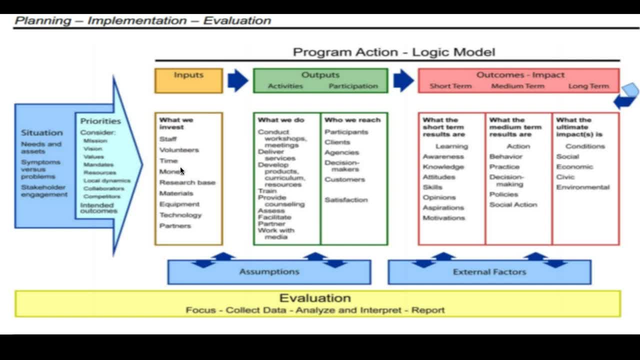 happening. So what are the things that are going in to this so-called process? okay, Once we understand our inputs, we're able to reflect on the inputs that are happening, And so we need to. we can then look at two types of outputs: our activities and our participation, what we do and 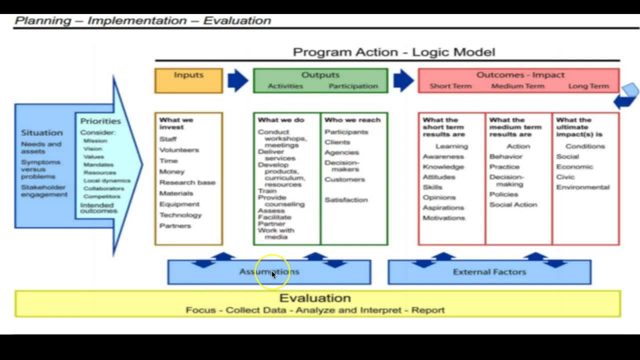 who we reach, And all throughout this process, we are making sure we check our assumptions And we're evaluating the work that we do by using focus groups, collecting data, analyzing and reporting, And so that's what's underpinning all of this. Once we've looked at our outputs, we then need 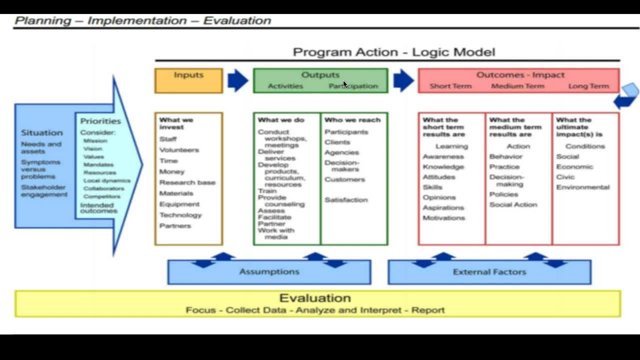 to look at our outcomes. Outputs are things that come out. Outcomes are things that we want, The goals that we want to reach right. Another way to think of outcomes is impact. What impact do we want to have? So how are our inputs relating to our impact? When thinking about our impact,